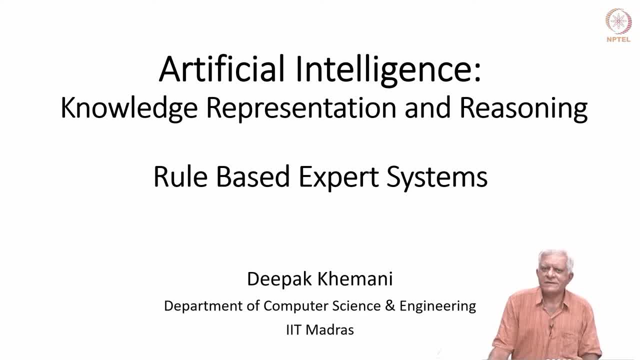 to order the clauses carefully. The idea on rule base system is is more general in that sense that you just give us the rules And we will write an inference engine which will run those rules. essentially, Of course, we will give you some meta level control. 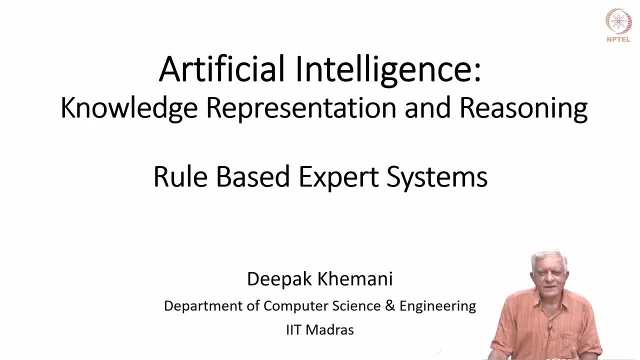 So we will look at something called search strategies, And once you have chosen that, then we will do the rest of the job, essentially, But the rules do not have to be written in a particular order or in a particular fashion, essentially. So let us start with that. 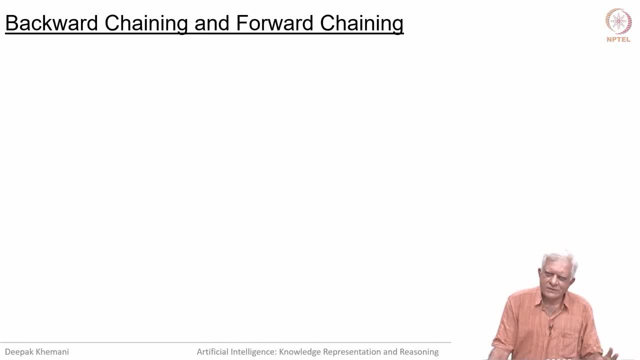 We have looked at backward chaining, we have looked at forward chaining. We have also looked at resolution method, which was a complete method, But for our current interest, forward and backward chaining is what we are going to be working with. So rules: they connect antecedents to the consequence. 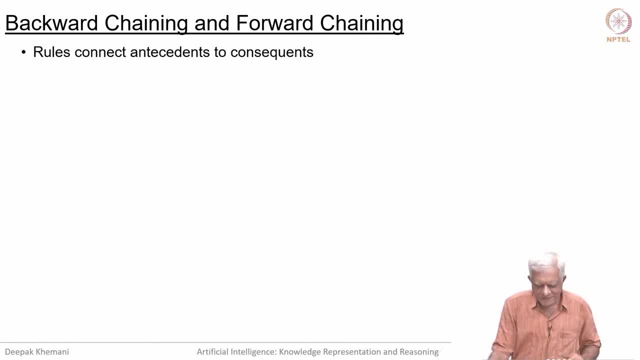 So that is the idea of a rule: If the left hand side is true, then the right hand side is true. essentially, We imagine the world described by statements in some language. In our case, it is going to be first order logic. 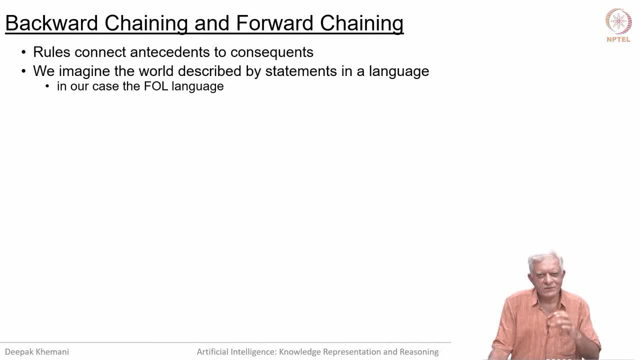 And then we will write rules Which will look at subsets of this knowledge base or look for patterns in the knowledge base. That is the idea of writing rules. essentially, The antecedent of a rule captures a pattern in the domain That if you are looking for a certain kind of pattern, then the rule will capture that. 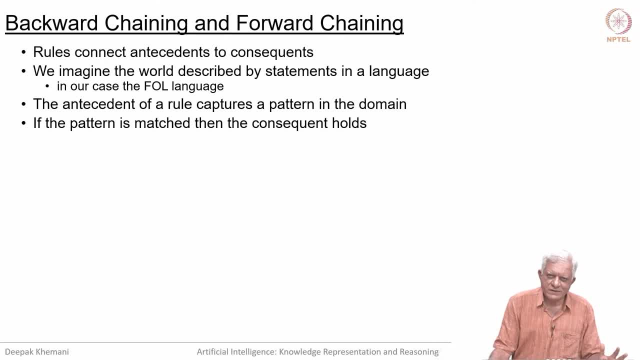 If the pattern is matched, then the consequent will hold true and if you are doing logical reasoning, Then you will note that the consequent is true. But we will see that the idea of rule-based systems is more general than just making inferences. 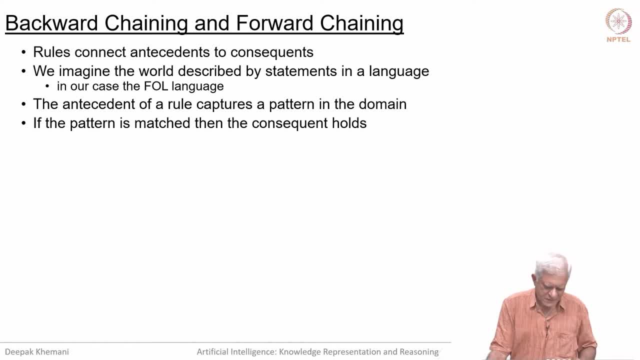 You can also trigger actions essentially, And this language that we are going to look at allows us to do that essentially. So backward chaining looks at the goal and it translates into the sub-goal, It repeats that process till the sub-goals match something in the. 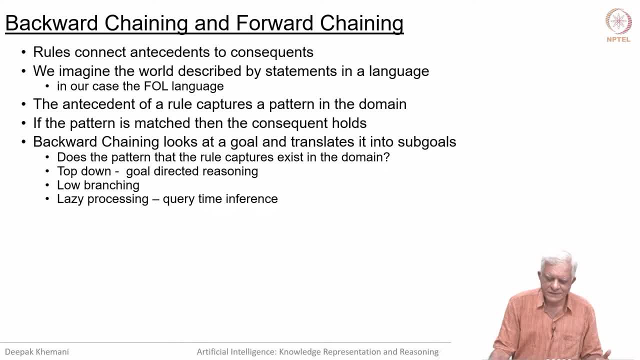 So backward chaining looks at the goal and it translates into the sub-goal. It repeats that process till the sub-goals match, something in the. So backward chaining looks at the goal and it translates into the sub-goal. It repeats that process till the sub-goals match, something in the. 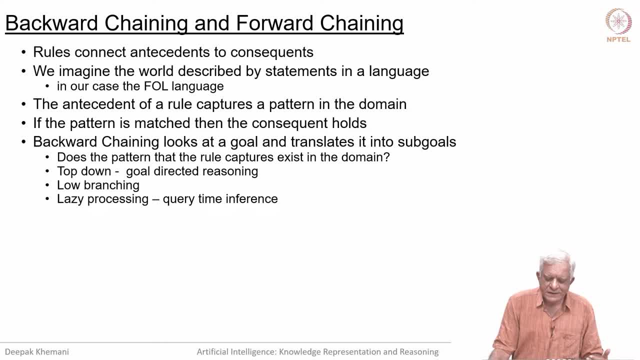 Knowledge base. Does a pattern that the rule capture exists in the domain? that is the question that we asking essentially. So if we have a goal and the goal has the antecedent, which is a pattern, and is that matched in the knowledge base? 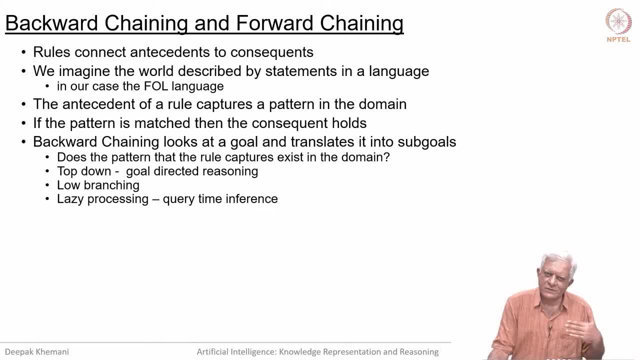 So it is a top-down process: From goal we are going to the sub-goals, towards the individual facts. if you want to say that goal directed essentially, It has a low branching factor because only the rules which have the goal as a consequent will apply. It is also lazy processing and you make the inferences. 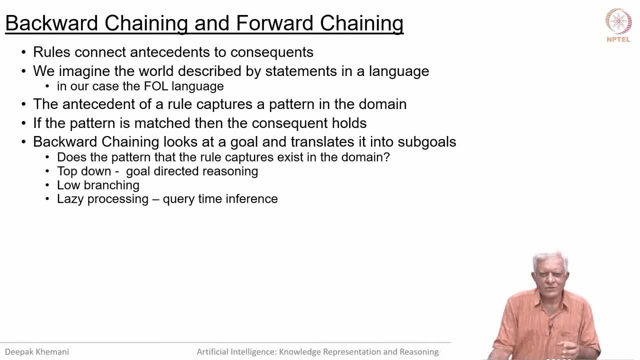 only at query time. When somebody asks that, is this particular goal true, only then you go ahead and make this inferences, which of course, means that it could take time also. On the other hand, forward chaining focuses on the pattern in the data and considers the 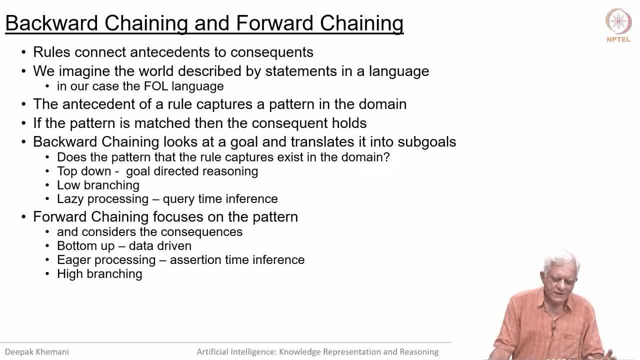 consequences of that pattern. essentially, It is bottom up, it is data driven. It looks at data and say, oh, I see this pattern and this is the action that I can take, or this is the inference that I can draw. By definition, it is eager processing as opposed to lazy. 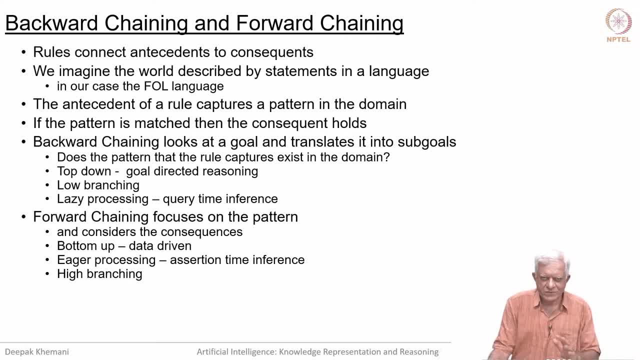 processing is that if you can make an inference, you go ahead and make it. You do not consider whether you wanted to make that inference or not, or whether it is leading to you to the goal that you have in mind or not. You just go ahead and make that inference. And that is why these 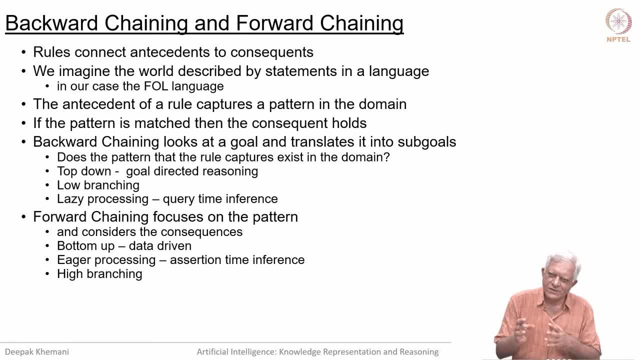 kind of methods. they need some additional guidance as to you know which of the possible inferences that we want can make. which one should you really make? essentially Because we are assuming that we can make only one inference at a time. It has obviously high 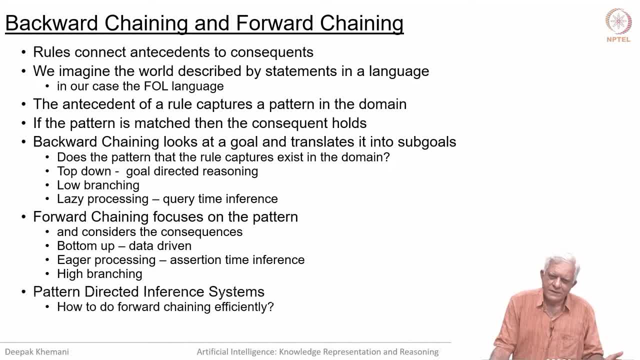 branching, because many inferences may be possible. Now all of them will be relevant to the goal that you are very interested in. So this field of forward chaining, data driven processing, is also called pattern directed inference system- That you look at patterns and based on that, you make inferences and 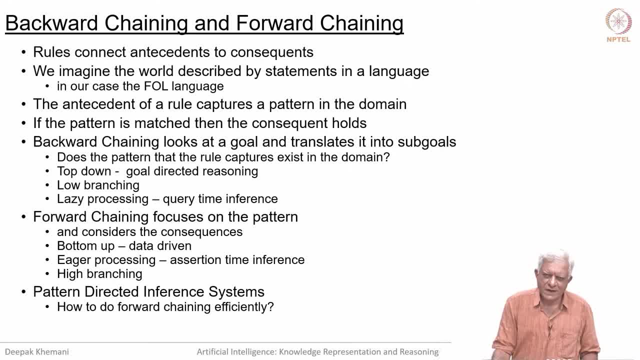 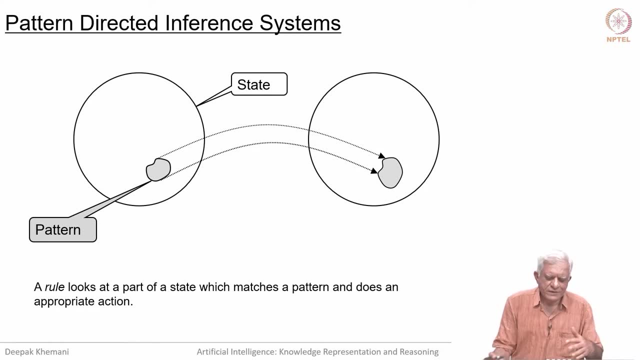 you proceed in this fashion. The question that we are going to ask today and address it is how to make forward chaining work efficiently. So that is the idea of a pattern directed inference system. So if we have some given state which we can also call as a knowledge base, then a rule, 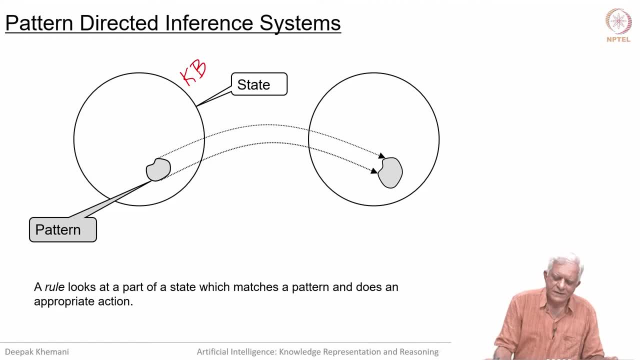 looks at a small subset of the knowledge base and does something, essentially Makes an inference, is the simplest thing that you can do, but you can do other things also. essentially, You can trigger some actions, for example, if you are controlling a robot and things. 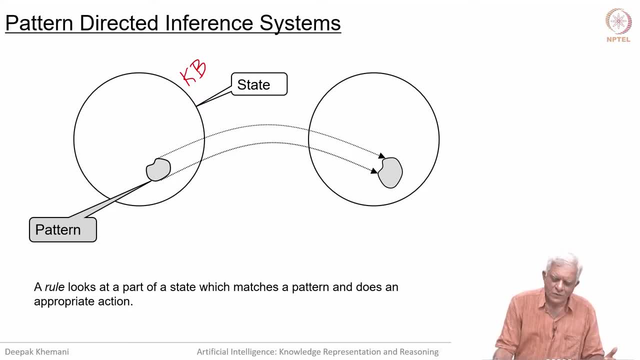 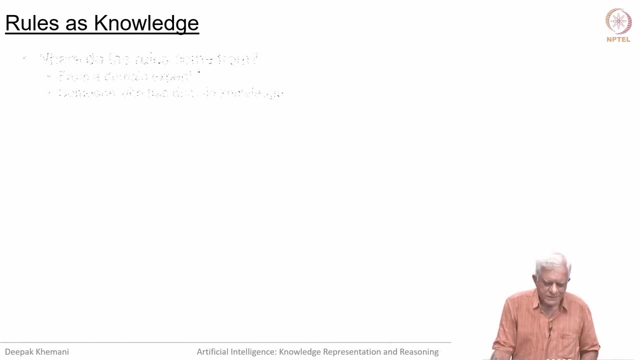 like that. So a rule looks like at a part of a state which matches a pattern and does an appropriate action, essentially, which is given in the described in the rule, essentially. So what triggered this idea of rule based expert systems is that: ok, fine, you are building. 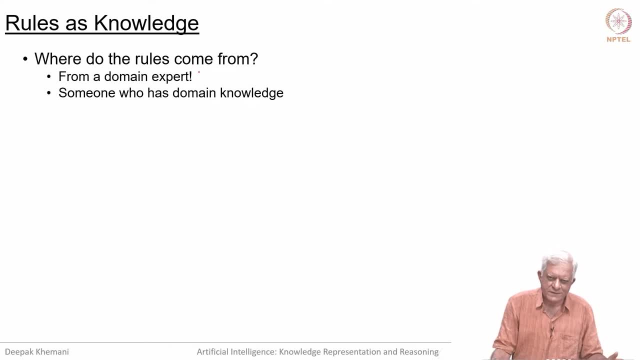 this system. but where do the rules come from? essentially So obviously, every time you develop some software, you have to somehow inject domain knowledge in that. essentially, Even simple things like sorting an array. you have to study sorting methods and decide: ok, this method will work in this situation, this method will work in this situation. and 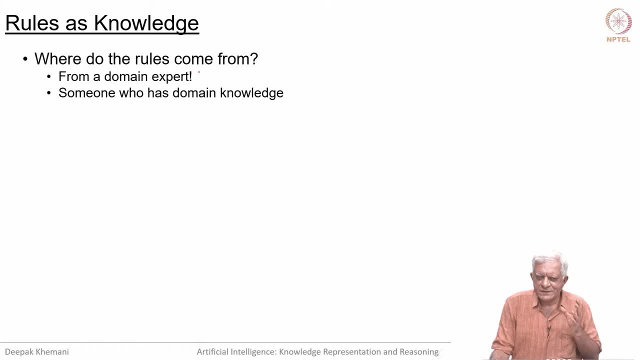 so on. So, some, somehow the knowledge has to be either embedded into the system, as it is done in individual languages, or it has to be expressed as in some form, as it is done in declarative languages like prologue, and the language that we are going to look at today, ops 5.. 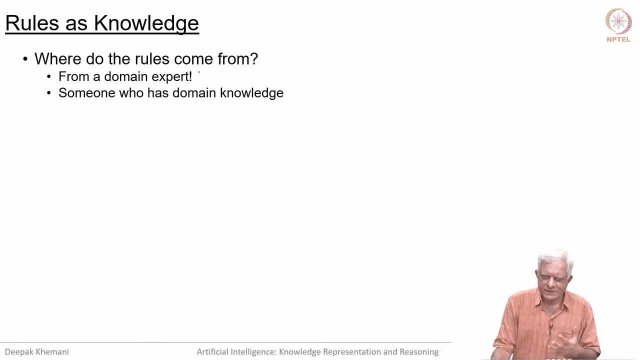 But the thing is that these rules have to come from somewhere. essentially, who knows about this domain that we are trying to solve the problem in? So let us call that domain domain expert who has this domain knowledge, and the idea behind rule based systems is to extract that knowledge. 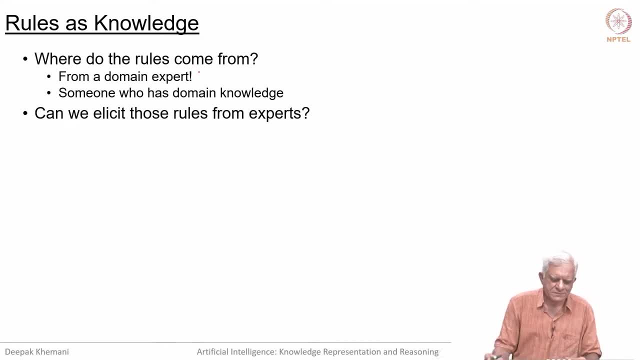 So extract that knowledge from the domain expert and put it into the system. So can we elicit those rules from experts. So the expert may be an expert in whatever domain that they are working on. and that is where the idea of rule based expert systems came up. 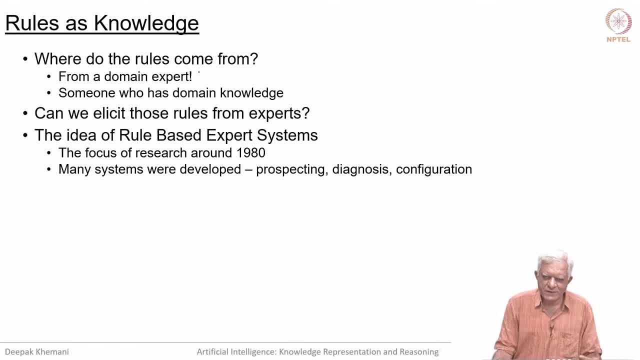 This was very popular around 1980, little before 1980 and a little after 1980 also, and many systems were developed. They were developed, for example, prospecting. So if you are a company which digs oil from the earth, then you have to, you know, dig. 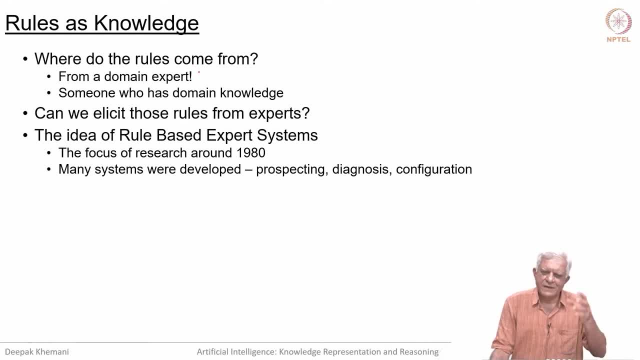 you have to, you know, search for where could oil be, do some study, make a well, dig it and see if you strike oil or not. So this whole process is so expensive that people feel that if a rule based system, people felt that if you, if a rule based system could, 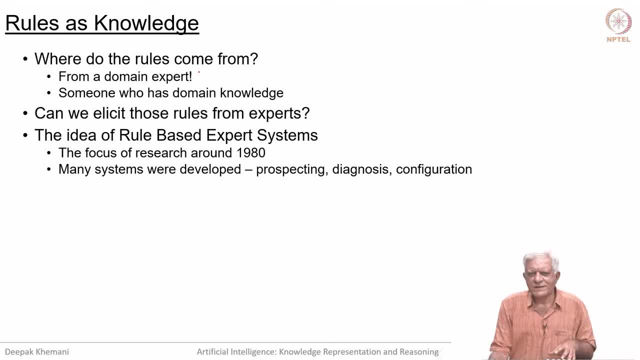 Give us a good idea of where to dig, then it would, you know, pay for its own development simply by the amount of money that it would save the company. So there was a system called prospector. maybe you should go and look at that. essentially, 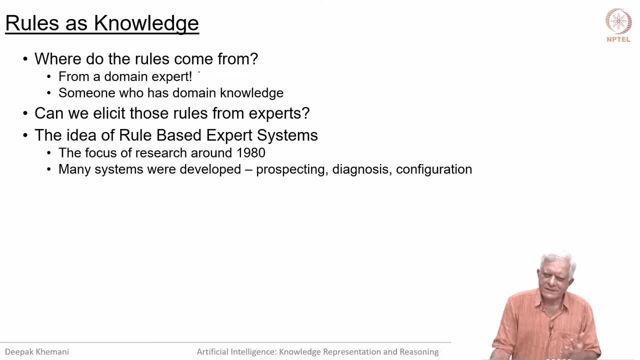 Another feature were people try to develop expert systems was in diagnosis- human diagnosis as well as machine diagnosis, because diagnosis is really pattern driven. you see a certain pattern make certain inferences. Diagnosis is complicated by the fact that it is not deduction. it is as we have discussed. 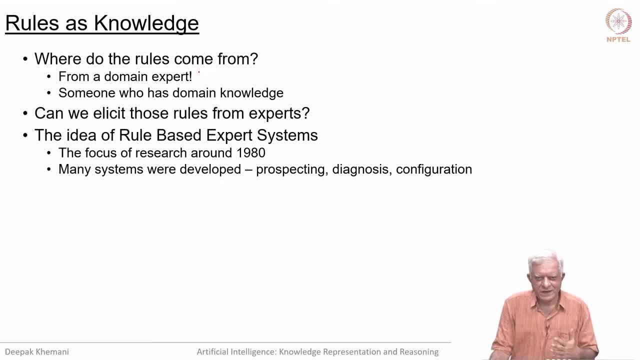 earlier. it is abduction, but nevertheless it is a very useful thing to have and therefore people have spent a lot of time doing diagnosis. So one of the earliest diagnosis systems was a program called Mycin. if you just look for this on the internet, you will get some information about it. 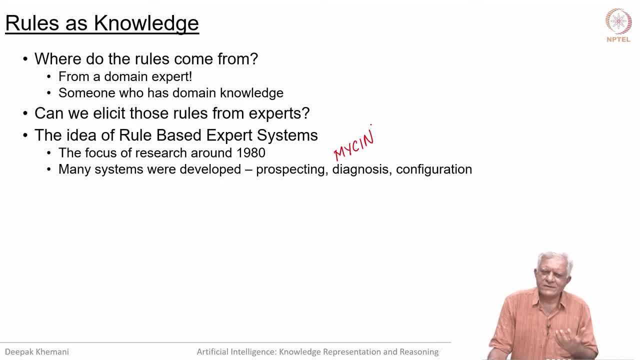 Because of the fact that it was doing abduction, it introduced a measure of belief or a measure of accessibility of its conclusions in the form of numbers, which were called as certainty factors. that, how certain are you that if you see these, these, these symptoms, then this: 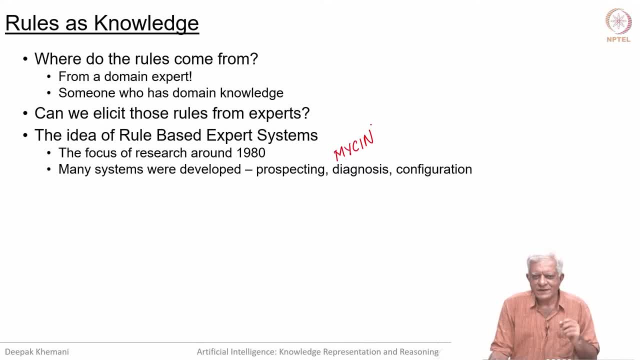 is the disease, Then the rule came with this: certainty factors and therefore you know you could at least try and evaluate, of all the possible hypothesis that you are making which one is the most likely one. And configuration. we had already mentioned that. you know they were used for configuring. 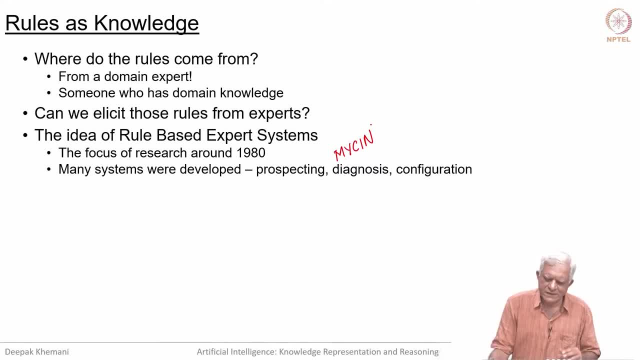 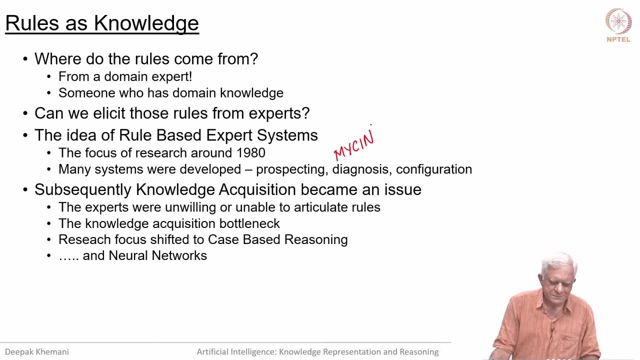 systems in this language and maybe we will look at that example very quickly again. essentially, What happened in After this rule-based expert system idea came forward is that people discovered that that that conceptually, it is a great idea that you go to an human expert elicit their knowledge. 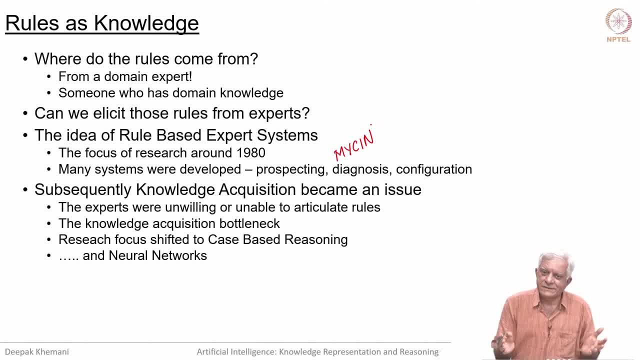 put it in a system and low you have a expert system. But it turned out as it turned out, the experts were either unwilling or they were unable to articulate the knowledge in the form of rules. So in those days the community had developed a lot of protocols. 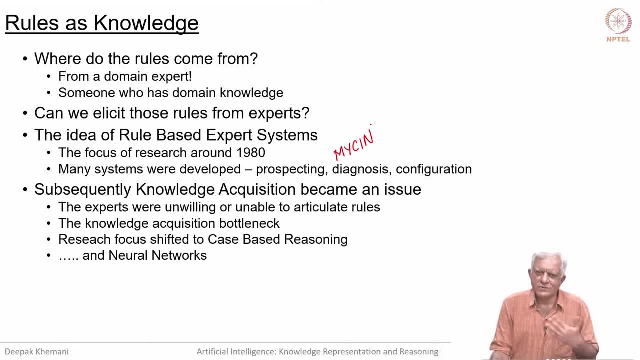 So the rules were developed, protocols which said that this is how you should extract knowledge. So knowledge acquisition became a big thing and people put in a lot of effort, So they would record interviews instead of asking the experts to articulate rules directly. 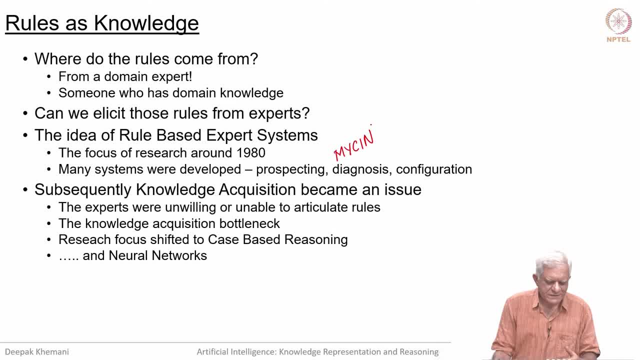 and then from that they would try to extract rules and that kind of stuff, essentially. But it was not easy and it became a bottleneck, So that was known as the knowledge acquisition bottleneck. What happened in the mid-80s is that people said that, okay, instead of abstracting these, 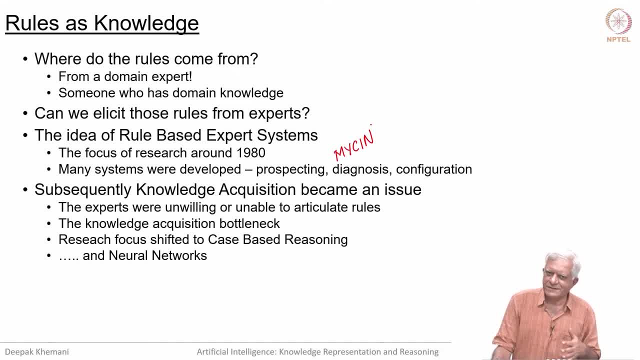 rules from experts, why do not we just store their entire experiences? And that gave rise to a whole new field called case-based reasoning, where every instance of problem solving was stored as a case. And a case had two parts: one was the problem description part and one was the problem. 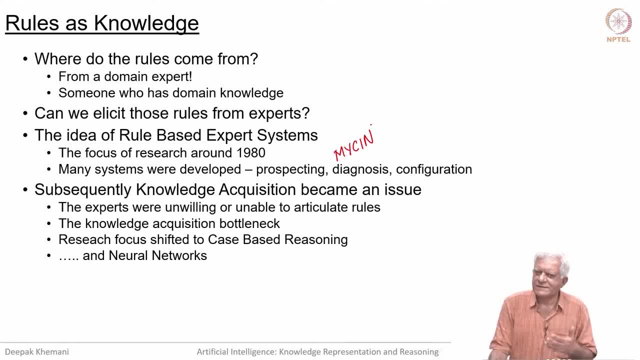 solution part. So if you could just store the entire thing as a case and then you had a whole repository of cases as experience grew, then when you see a new problem to solve you match the problem with the problem part of your cases. 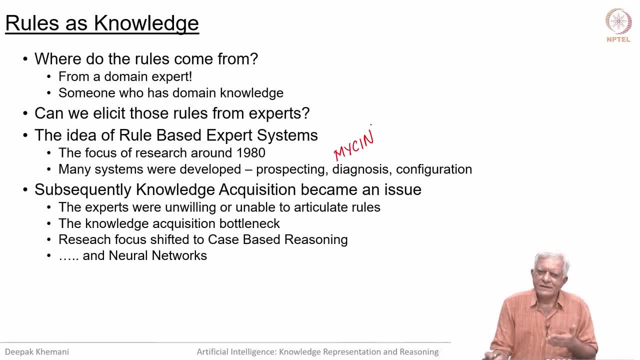 So retrieve the case which matches best the problem description, take its solution description, maybe adapt it a little bit to the current problem and you have a problem solver there. It is also knowledge-based. it is just that the knowledge is not articulated explicitly. 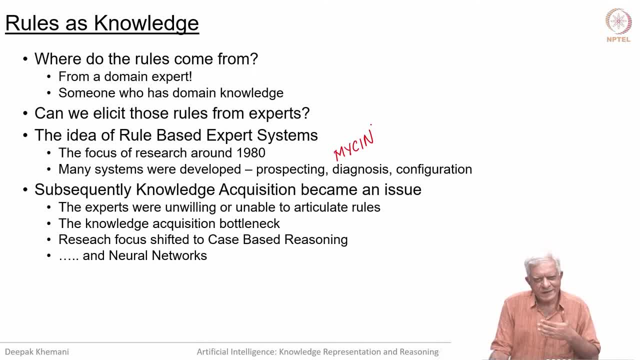 in the form of rules. the knowledge is stored as direct experiences from which you would eventually would have derived the rules And case-based reasoning says: let us use those experiences directly, And it was also a very successful way of solving problems and a lot of industrial systems. 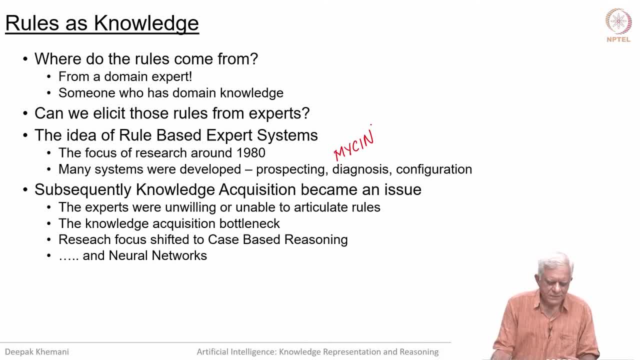 were developed which were based on case-based reasoning, And of course in the mid-80s Rumel Hart and then company again gave us the backprop algorithm for neural networks. So it kind of the interest in neural networks came back and since then we have not looked. 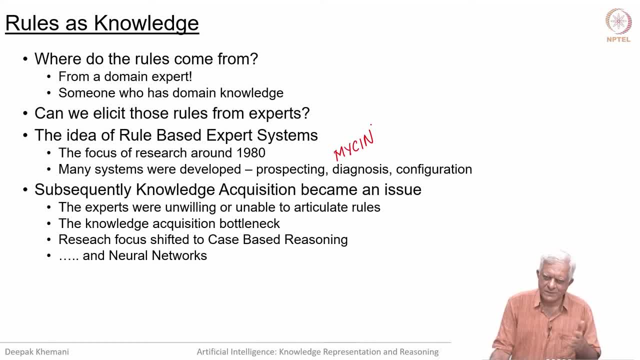 back 84,, 85,, we got the backprop and sometime early in this century we got this algorithm for deep learning, And since then neural networks have been a focus of many people who work in AI. But the businesses had spotted an opportunity and they struck to the idea of rule-based 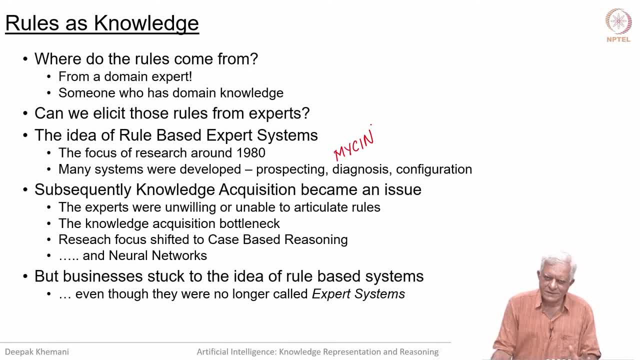 systems. Even though they would not call them expert systems, they were definitely a useful way of implementing software and typically in businesses where you have something called business logic- the idea that the managers in the business could articulate that logic and put it into their system- 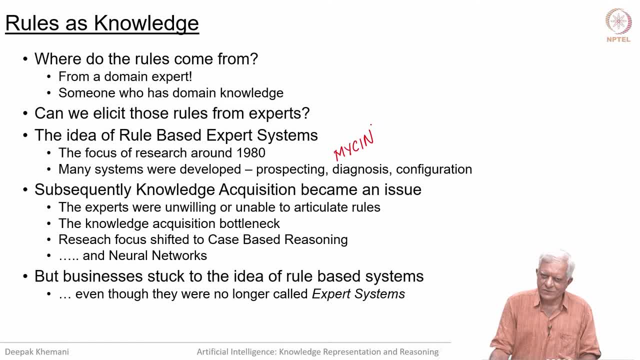 And some system would actually run as a web. So many systems would be on the schematics, the processes of program. it was very appealing to them, essentially because they did not have to go to a software firm every time they tweak something, Because if you are doing programming in a procedural language then a lot of the stuff. 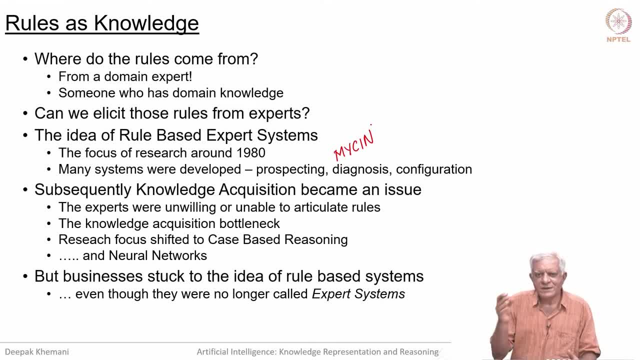 that you lot of the knowledge that you are putting in is embedded in the code. essentially, The idea of declarative programming is that control is different from logic. So if you can express the logic separately and leave the control to the machine, then 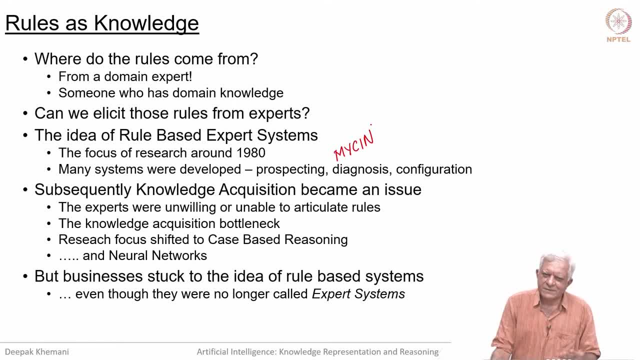 we have a different paradigm of programming, and that was eminently suitable for people who worked in business, because for them, expressing the logic itself, and maybe tweaking it as they experimented with their system, came quite naturally. But they were not called expert systems any longer, they were just called rule-based, rule-based. 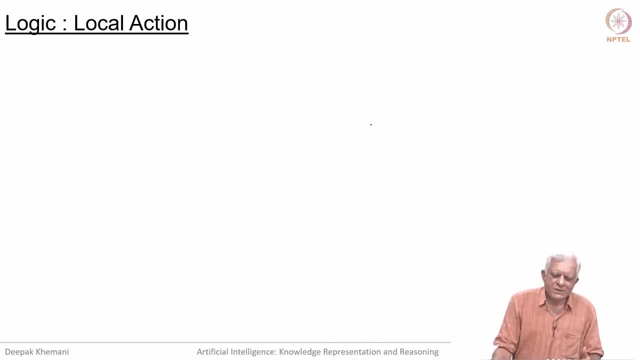 systems. Now, one thing about logic is that you may have a large knowledge base, you may have a large description of the world, but making inferences is something which is local. it is a local action that you do not look at the whole knowledge base to arrive at a conclusion. 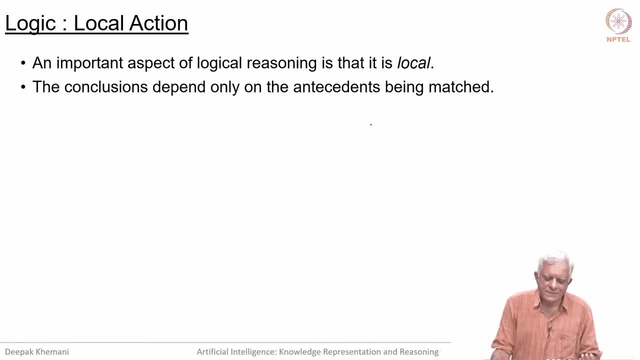 you only look at a part. essentially So the conclusions depend only on the antecedents being matched. essentially So, if you have a rule and if you can find the antecedents of that in the knowledge base, then you can go ahead and make the conclusion. 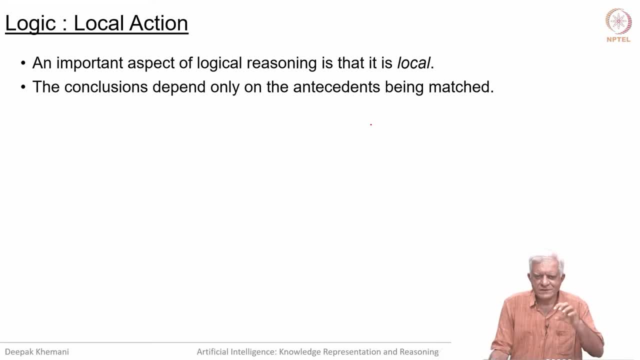 So in that sense it is local in nature that you look at local patterns and you make local inferences From the complexity purposes. that makes life better. So one does not have to consider the entire knowledge base essentially. So, for example, if you have looked at algorithms for state space search, they treat the whole. 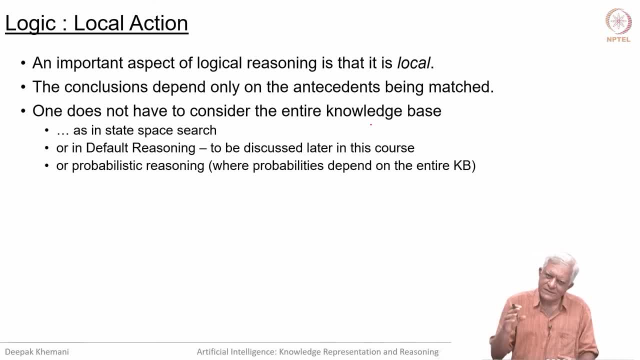 knowledge base as a state and say: from this state I can go to this state, and from this state I can go to this state, and so on, and so on. Or if you look at something called default reasoning, which says that, for example, you: 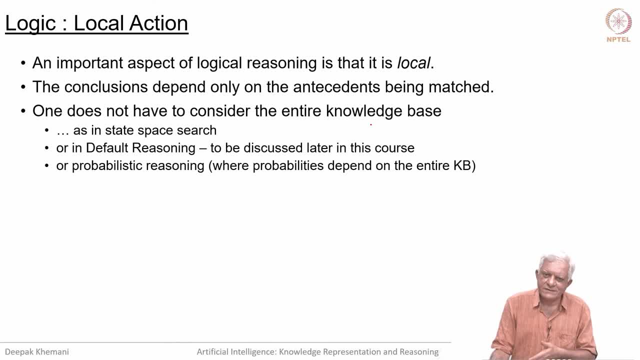 might want to say something like: if X is a professor, then X has a PhD, unless something, something, something. There may be eminent people who are professors and who do not have a PhD, but you want to make that inferences that the professor in general have PhD. 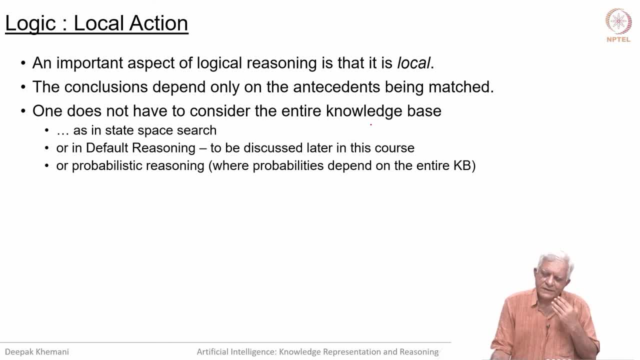 Now, as we will see, we will look at various axioms. Ok, There that at default reasoning, as we go along To make default inferences, you have to look at the entire knowledge base. So, complexity wise, that goes up essentially In a similar fashion. 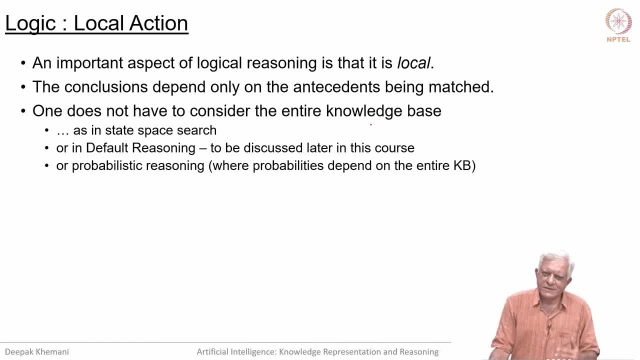 probabilistic reasoning will also depend on knowledge base, because the probabilities will come from the data and the knowledge base. So rule based systems exploit the locality of action essentially, which is true of logic in general. Forward chaining actively considers patterns in the domain and it says that if I can see this pattern I can do this action. 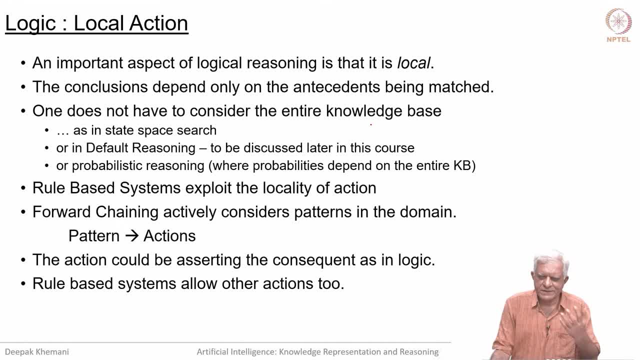 The action could be making an assertion, as in logic that this, that if this pattern is true, then this consequent is true essentially, but it can do other things also, As I said, that you can have any A kind of action. So if you see this pattern, do this and this do this could include making. 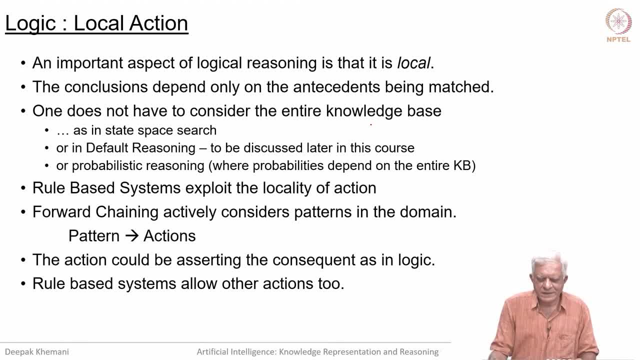 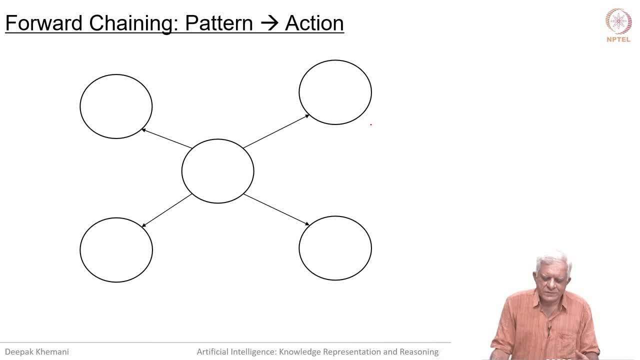 an assertion, So in that sense it subsumes making influences. So if you are in a given state, then you can maybe spot many different patterns in that state and therefore many rules are applicable. Okay, And you may want to choose one of them. So a state is a set of sentences in some language. 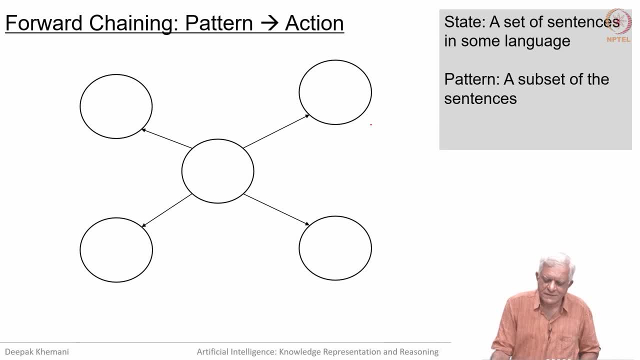 So it is a knowledge base. in our case, language is going to be first order logic And the pattern is a subset of those sentences in in that knowledge base And a move or an inference or whatever you want to call. it says that if you see a pattern, then you do some action. 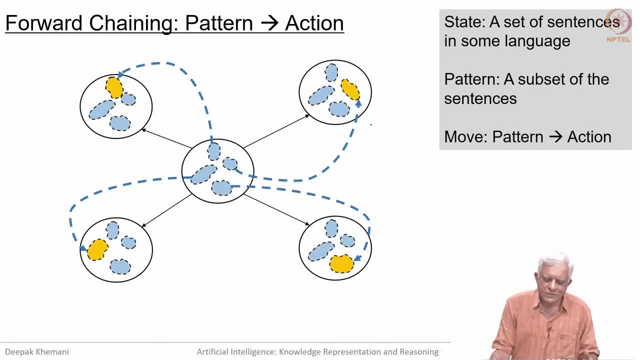 essentially So. it could be that you could, in this example, see four different patterns and therefore do four different actions. The key point, of course, will be which of those four choices will you make, and that is where the effectiveness of the system will. 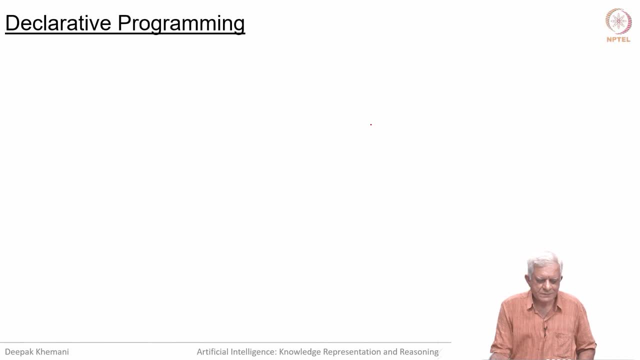 lie. We have already been speaking about declarative programming, So let us do a quick kind of a recap of this. A rule associates an action with a pattern in the state. essentially, In the language that we are looking at, a rule is also called a production. A production- 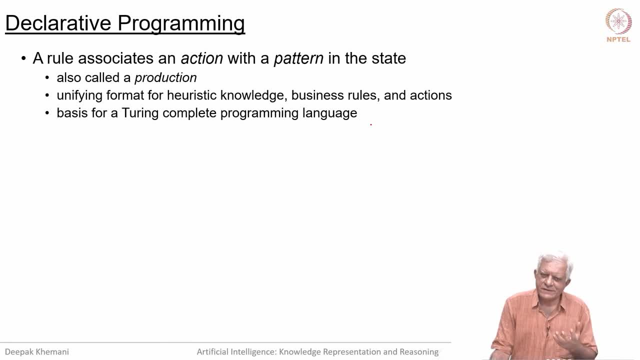 or a rule. it unifies different kinds of knowledge into one form. It can be heuristic knowledge that if this is a pattern, then this is the right kind of action. It can be business rules like if this is the, let us say- description of a loan seeker, then this person is eligible. 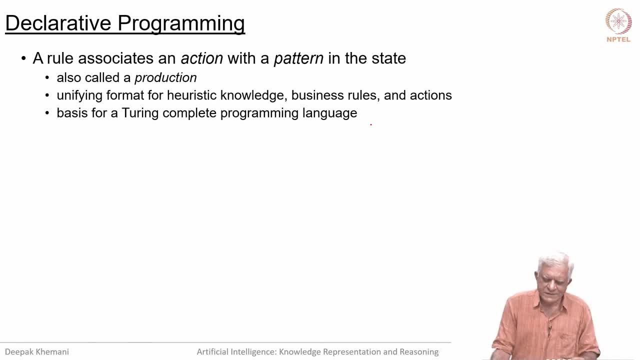 for a loan. So it could even be actions in a programming language, essentially, as you will see, So it is. it turns out that these rules are enough to define a complete programming language which is Turing complete essentially. So, just like prologue is Turing complete, this.